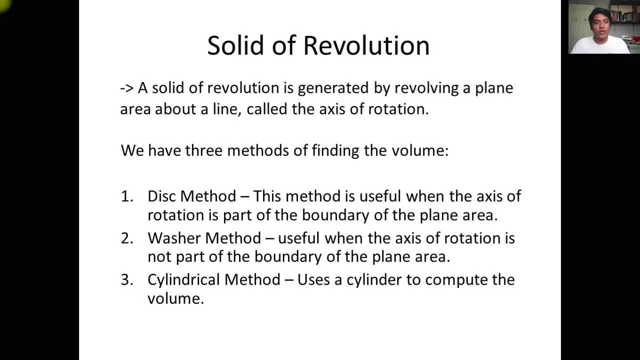 the intersection of the curve with respect to that axis of rotation so in other words if we have two uh if we have two curves that intersect then we're going to get the volume vector intersection so we're going to retake the axis so if we are calculating the area we are only getting a sketch of a two-dimensional uh two-dimensional uh graph but in solid earth revolution we need 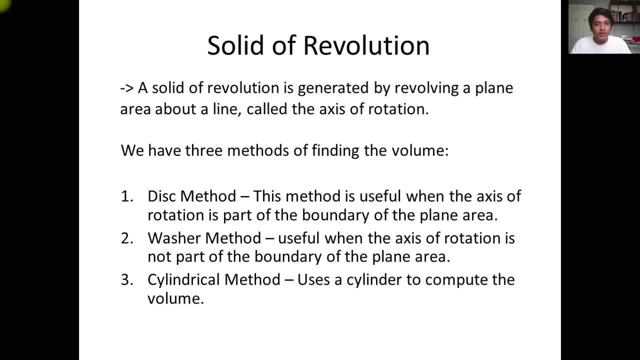 to be imaginative of uh what will be the uh shape 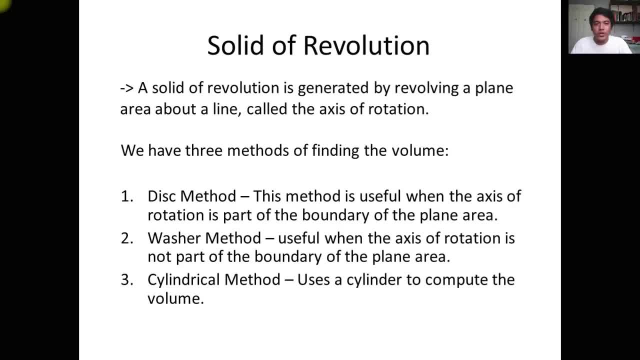 or the outcome of these two curves when we rotate it in a certain axis so we have three methods of finding the volume number one we have the disc method the disc method is useful when the axis of the rotation is part of the boundary of the plane area later you will see okay uh we have a curve we have one curve and it is bounded on a certain axis of the xy plane so it is 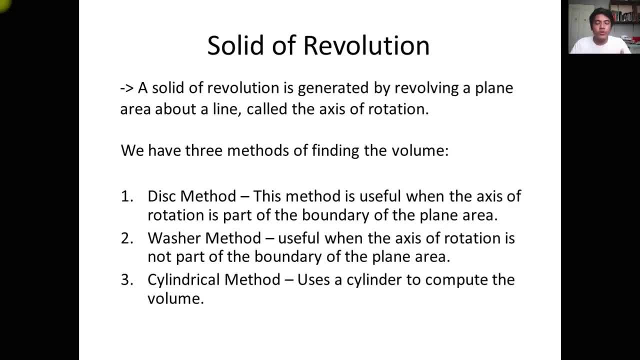 more most uh more easily to use more easy to use the disc method okay to find the volume of that plane area so the washer washer method it is useful when the axis of rotation is not part of the boundary of the plane area for example we have two curves and these two curves are not actually bounded by the x or the y so they have a specific boundary wherein uh they form a boundary not 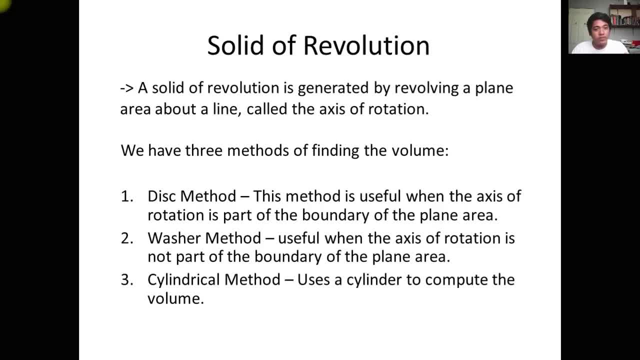 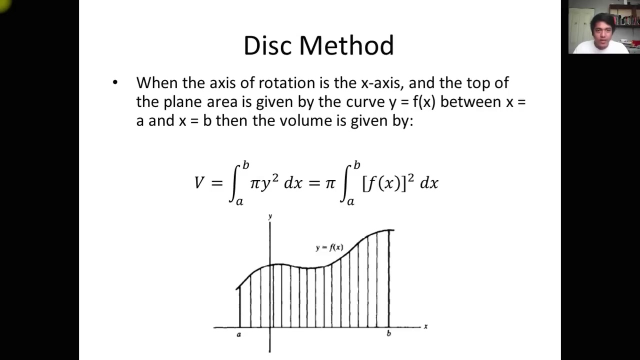 touching the x and y so what are we going to do is to use the washer method in this water washer method we have an outer radius minus the inner radius okay so we're going to use that formula we will be forming a washer type of a shape that has a inner radius and outer radius later we will see that so number three for cylindrical method from the word we're going to use cylinder to compute the volume of the solids of revolution okay let's start so for the disc method okay for example we have here y is equal to f of x okay and it is bounded by the 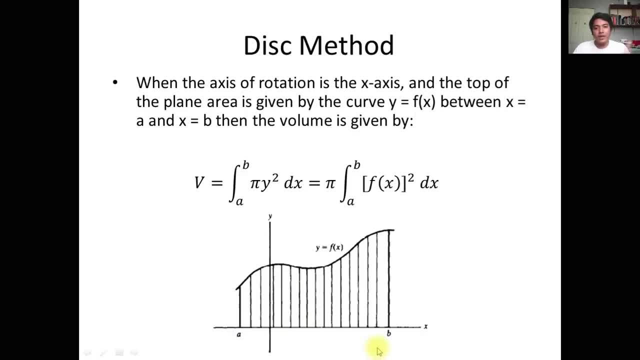 x-axis here from points a to b we can calculate okay the volume of this uh curve rotated about the x-axis of the cylinder so we're going to use cylinder to compute the volume of the solids of x-axis so meaning this is the curve okay this is the limits a to b so we know that we have an area here so to get the volume the problem says we are going to rotate it with respect to x-axis so if we rotate this with respect to x-axis we will be forming a three-dimensional figure of this plane so if we have this kind of uh plane uh when the axis of rotation is the x-axis and the top of the plane area is given by the curve y is equal to f of x between x is equal to a and x is equal to b that's the limit but then the volume is given by b is equal to the integral of pi y squared okay where y squared is actually the function here y is equal to f of x only squared so dx so if the axis of rotation is if the problem says that the axis of the rotation is on x-axis or this method you'll have dx here if it the axis of rotation is on the y-axis you'll write uh dy here so that is pi y squared dx so in other words we can background pi so we have now pi integral of f of x simply that is uh the f of application is fuck. 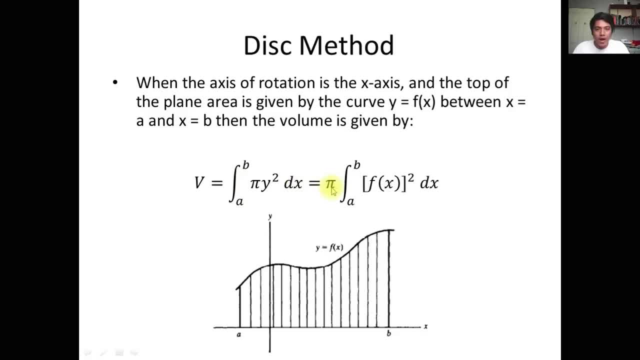 So we have now pi integral of f of x simply that is uh the f of x squared the x so we can ways to contract pi so we have now pi integral of f of x certainly that is uh the f of x squared the f of x squared the x so we're now going to work on the diveiche. 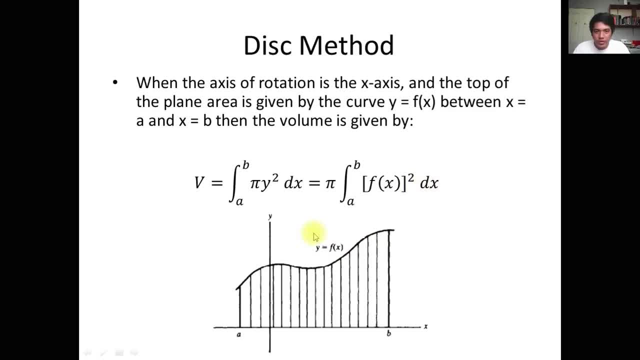 But we have also uh look at the your low numbers of the two second everyone's or the other up guru dx so we need to express the equation in terms of x because it is rotated about the x-axis so 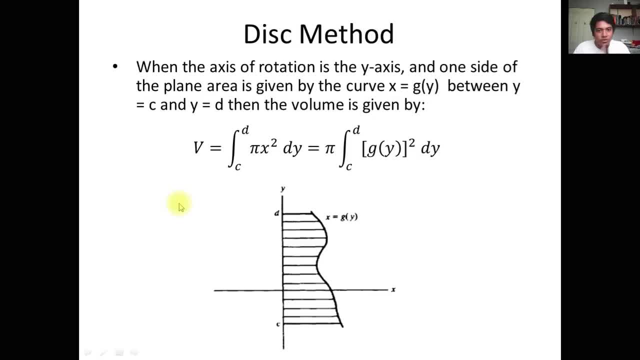 we have this formula how about if the rotation is on the y-axis so for example we have now a function of x in terms of y so we have this graph okay this is bounded on the y-axis with limits from c to d so what will happen is that uh in this problem the axis of rotation is now the y-axis so we're going to rotate this plane with respect to y-axis what do i mean to rotate to rotate 360 degrees so we will form again a 3d three-dimensional form of this figure so uh to calculate the volume we have b is equals to uh the integral of pi x squared x squared because this is expressed in terms of x and as i've said this is this rotation has an axis of rotation in the y-axis so therefore we have to have dy here okay a while ago we have 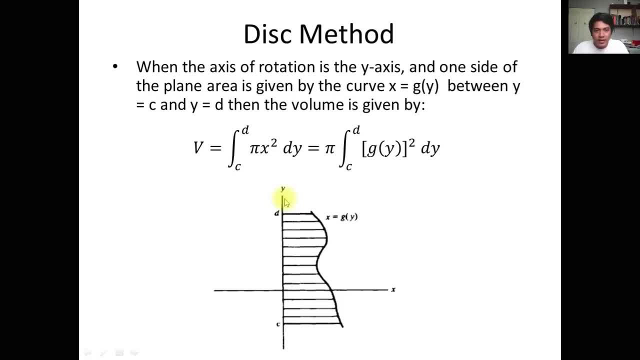 dx because the axis of rotation is at the x and here dy because the axis of rotation is at y axis take note that this dy and dx is only applicable in this method 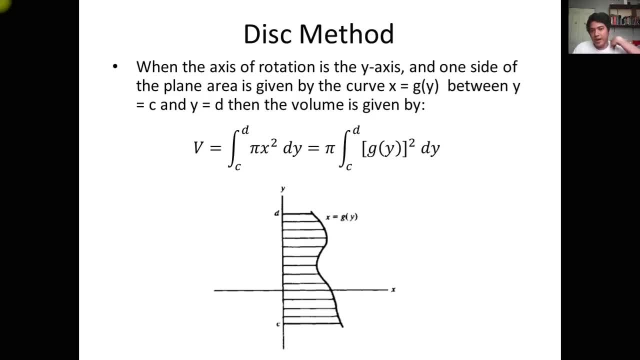 in the succeeding method the other two the washer and the cylindrical method so it's the opposite so if the axis of rotation is on the x-axis you're going to use dy and if the axis of rotation is on the y-axis you're going to use dx this is an exemption the disc method when we say the axis of rotation is on the y-axis then we have to use dy okay so we have pi integral of g of y the function of 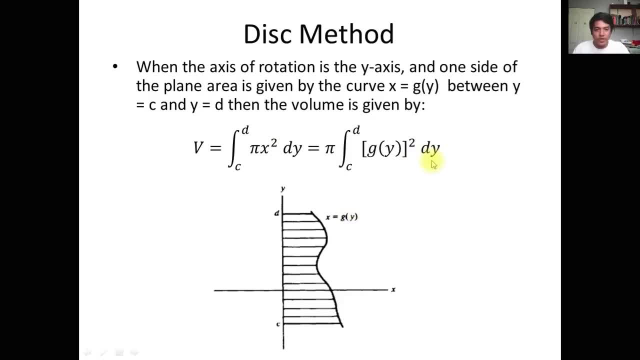 uh x with district uh in terms of y squared dy this is basically the same formula so it is the here we have dy so we have to express the function in terms of dy in order for us to integrate the function c to d is the limits okay and c to d lies beyond the y axis okay so that is for the 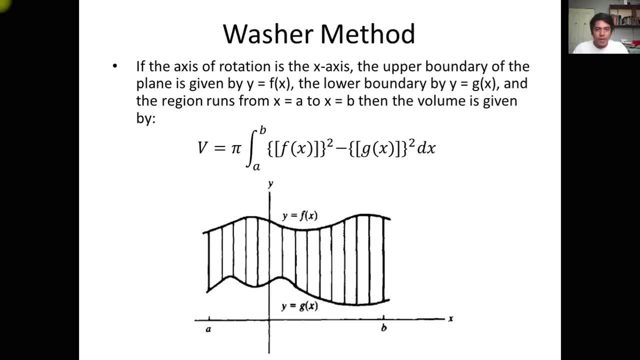 disc method how about for the washer method so for example as i have said a while ago we will be using 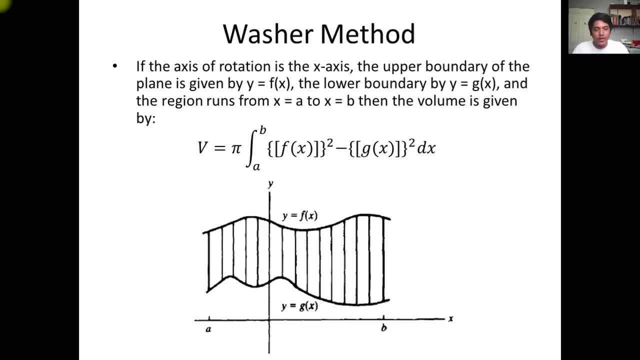 uh we have two planes bounded okay and they are not they they're bounded or their boundary is not actually involving the x and y so the area of their uh bounded area is not on the x and y so we're going to use the washer so called washer method so if the axis of rotation is the x-axis the upper boundary of the plane is given by y is equals to f of x represented by this figure the lower boundary by y is equals to g of x represented by the lower curve here 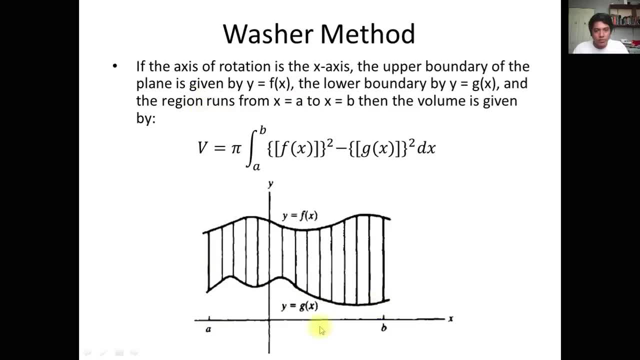 okay and the region runs from x is equals to a to b then the volume is given by this formula 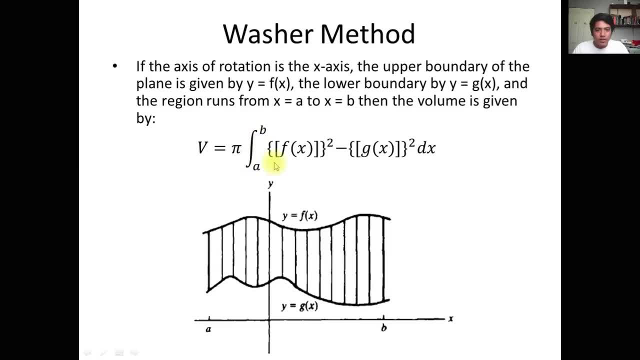 so what is this formula b is equals to pi the integral of f of x squared okay 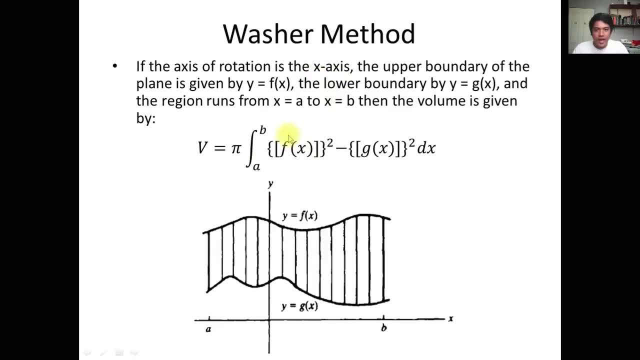 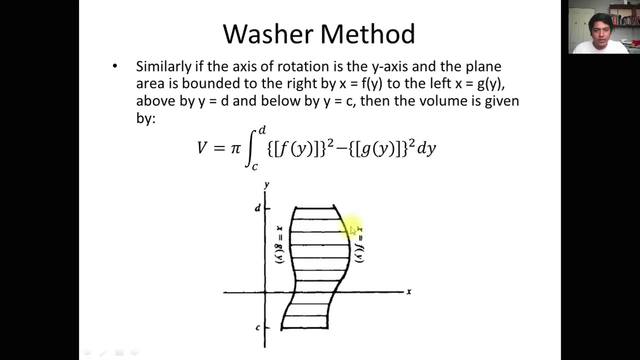 okay this is the rotation in x axis so my mistake so you have to still use dx for this okay because the rotation is on the x-axis the washer method so f of x squared minus g of x squared okay so uh what is this f of x squared minus g of x squared is actually the outer radius minus the inner radius of a washer figure the washer you can think of it as a three-dimensional uh uh a ring okay or uh what do you call this a a torus i don't know but uh that's the that's the figure so we have the outer radius squared minus the inner radius squared so then the volume is given by this formula so remember that the axis of rotation is on the x-axis so similarly if we are going to have this kind of function okay and the axis of rotation is the the y-axis we're going to use this formula okay b is equals to pi integral of from c to d fy of squared minus g y squared dy okay so the same method so you all you have to do is just remember this formula and make sure you know the axis of rotation again if it is on the y-axis we have to include dy here okay so again if for washer and uh we call this disc method so if the axis of rotation is x-axis we'll have dx here if the axis of rotation is y-axis you have you will have dy here and you're going to express all of inside of the integral in terms of dx or x for dx in terms of x for dy in terms of 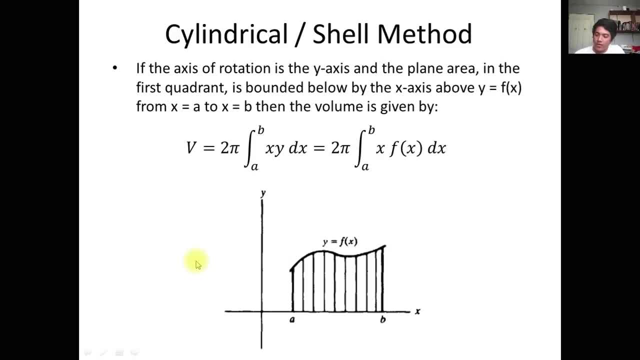 one okay so we have the cylindrical and shell method so for this if the axis of rotation is the y-axis okay so we have the y-axis here then definitely that's the opposite of what you will write uh for the integral here so if this if this is the axis of rotation is y-axis then we're going to have dx here oh and the plane area in the first quadrant is bounded below by the x-axis above so y is equal to f of x from a from x is equals to a to b then the volume is given by the 2 pi okay the integral of from a to b of x y dx if this is axis rotation in terms of y-axis so we have to include dx here equals 2 pi integral of from a to b of x f of x dx so we can express this simply this term of y into simply f 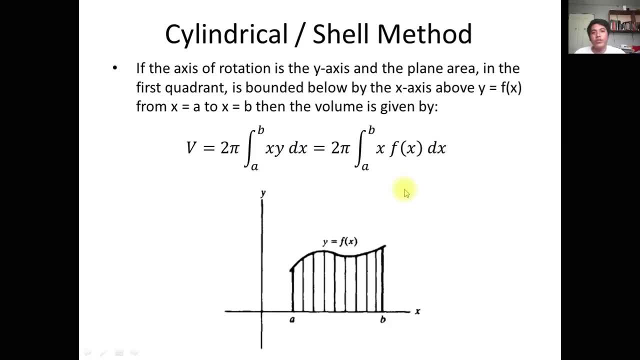 of x right so the cylindrical or shell method uses the method of the cylinder wherein we can think of this as x y as the radius for x and the y as the height of the cylinder so we have to find the radius of the cylinder when we draw a cylinder in this problem and we're going also to find the height of the cylinder so you can think of it always as the radius and height okay so you have to find the radius of the cylinder as well as the height in order for you to use the cylindrical or shell method and of course as i have said a while ago if you are going to use cylindrical or shell 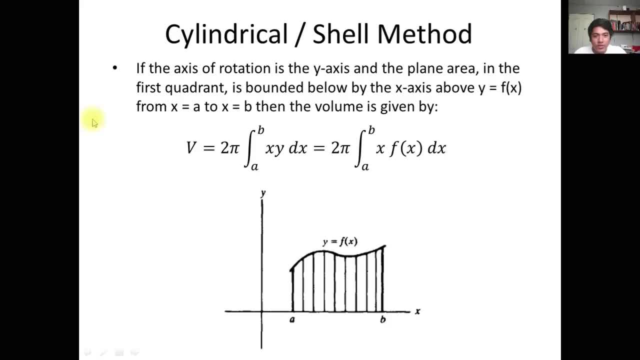 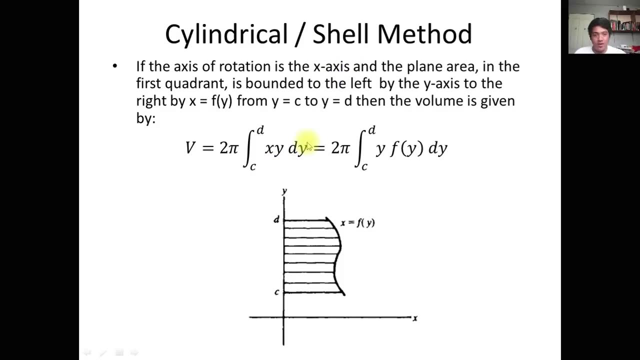 method if the dx or dy here will be determined by the axis of rotation if the axis of rotation is the y-axis so you have the x here so if you have an x-axis of rotation okay you have dy here 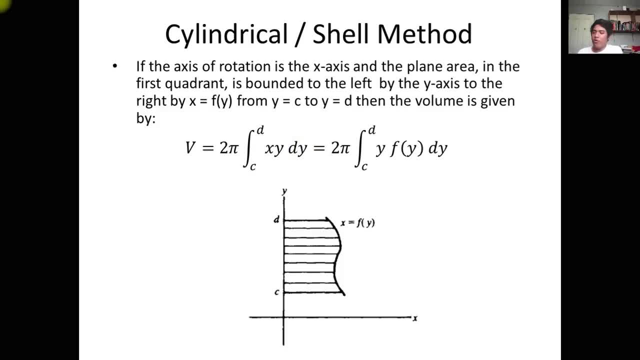 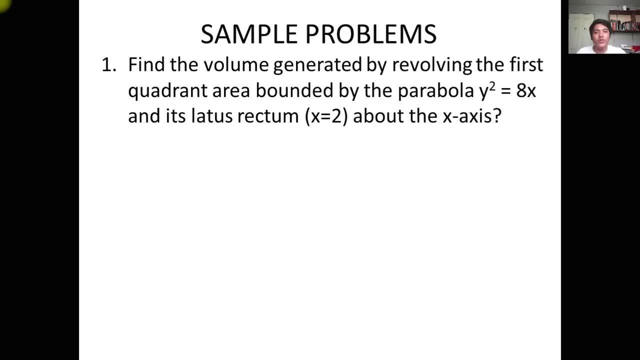 okay so now i hope you have taken notes of that formulas as we are going to solve our problems here okay so for number one we have to find the volume generated by revolving the first quadrant area bounded by a parabola y squared is equals to 8x and its latum rectum uh latus rectum uh x is equals to 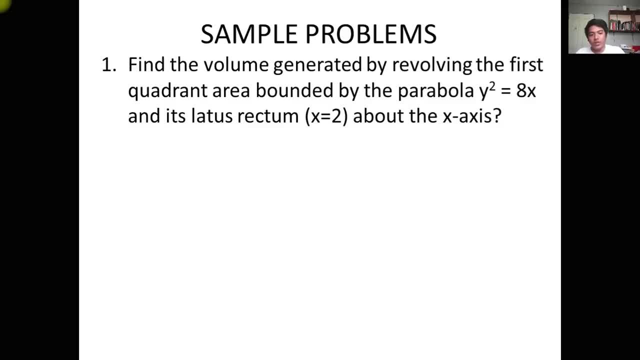 about the x-axis so what is the volume so first what are we going to do in order for us to solve these problems involving in calculating the volume of the uh the solids of revolution we 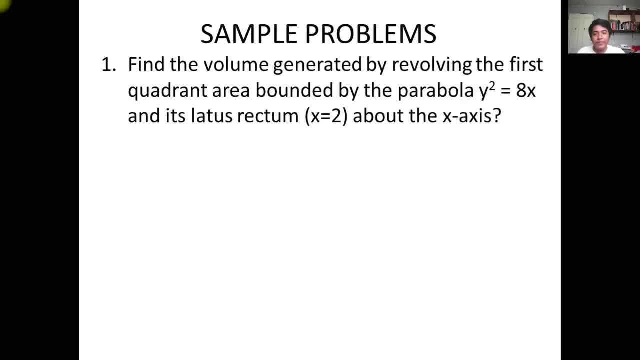 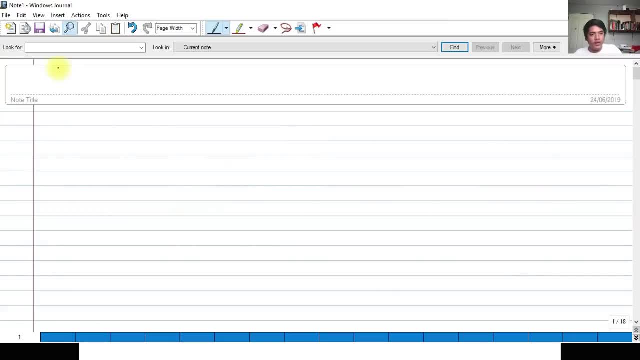 have to graph first the the uh the curves so we have a parabola y squared is equals to 8x so we have one here so y squared is equals to 8x so this is a parabola opening 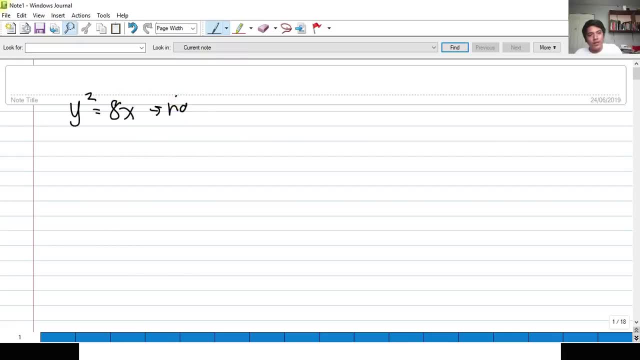 to the right okay so with a vertex zero zero vertex here is zero zero or at the origin so it has a latus rectum it's given x is equals to four so the problem actually is asking us find 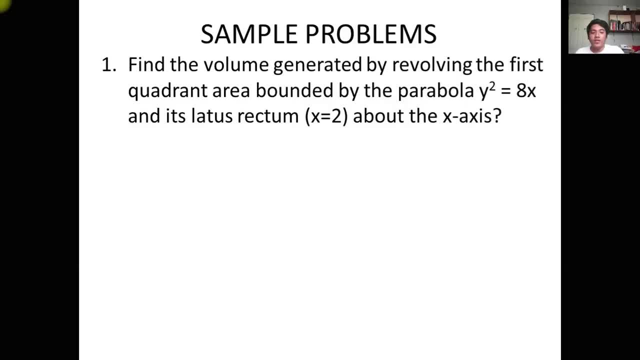 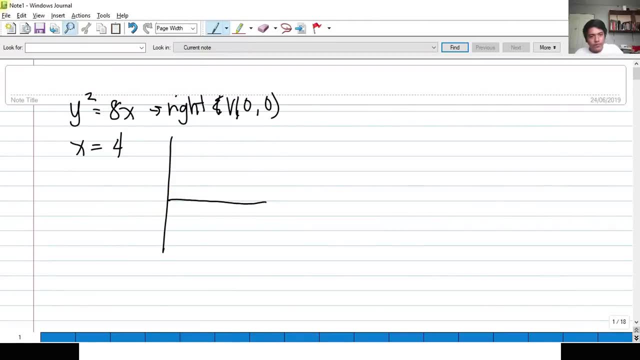 the volume generated by revolving only the first quadrant so because we know that if we're if we wish to graph our curve so here is our origin we have a parabola opening to the right oh oops let me just redraw this i'm so sorry i'm not really good in terms of uh sketching so i'll but i'll try my best 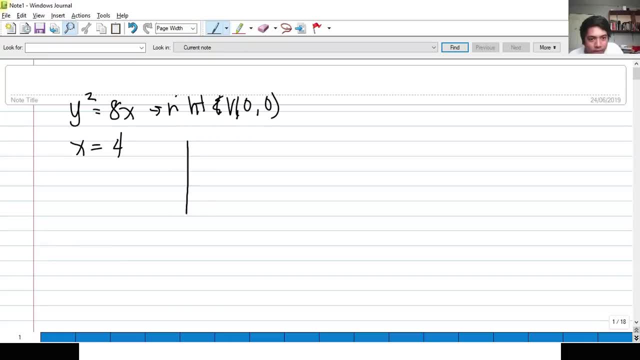 i'll try my very best so we have here the x and y so we have a parabola here opening to the right so this will now be our parabola 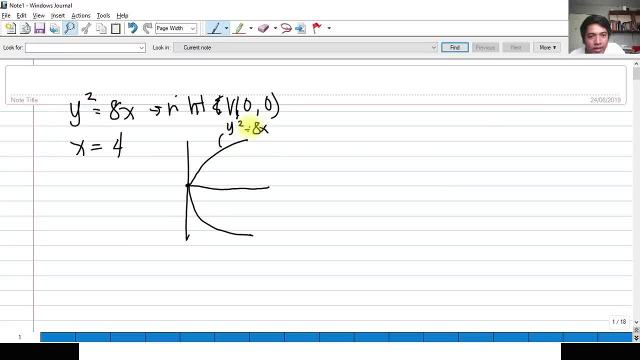 so this is y squared is equals to 8x and its latum rectum latus rectum is x is equals to four let's say that this is the the line through which that is the latus rectum of our curve so the problem states that we have a parabola opening to the right so this will now be our parabola 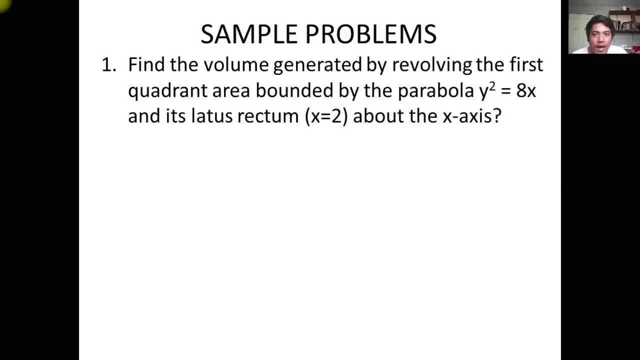 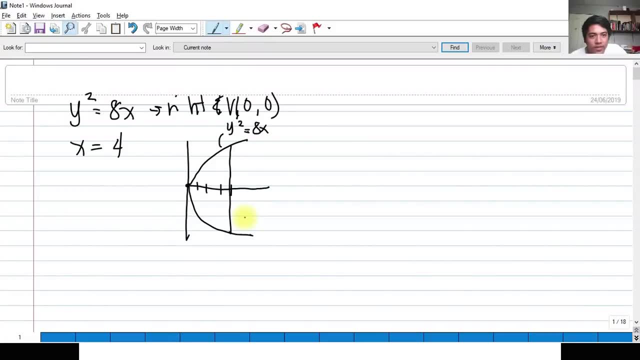 we have to revolve this parabola in the first quadrant area only so uh about the x-axis so if it's about the x oops i'm sorry the latus rectum is two so yeah so we have here again to redraw this so the latus rectum is only two so let's say this is the latus rectum x is equals to two x is equals to two okay so for the first quadrant only about the x-axis so we're going to rotate the x-axis okay and see what will be the form of this uh bounded area okay of the y squared is equals to 8x and its latus rectum so our figure simplifies as this so we only have to get the 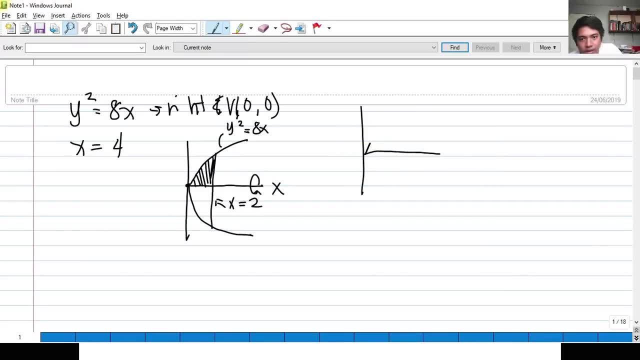 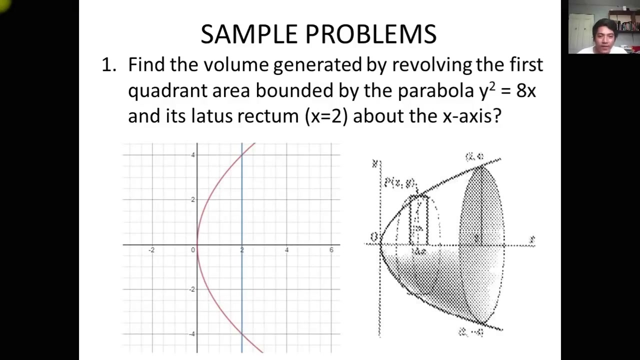 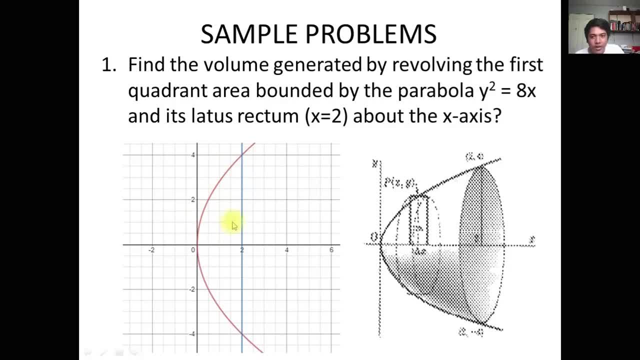 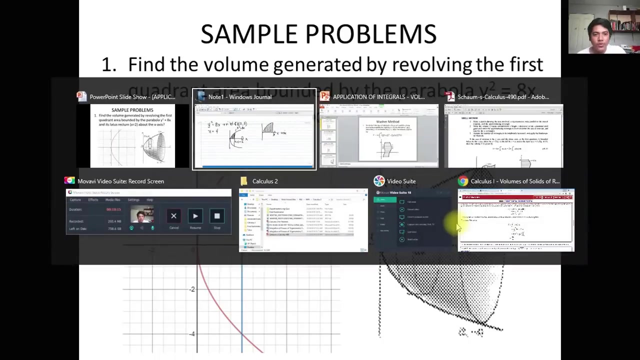 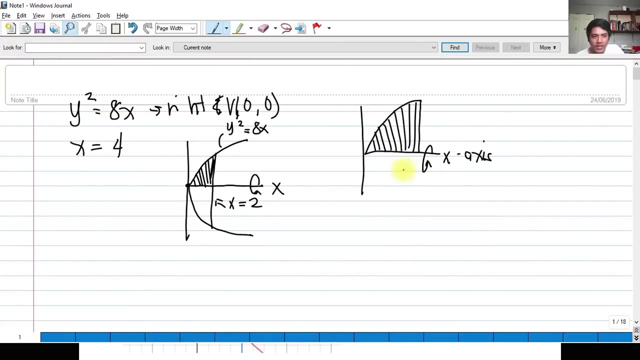 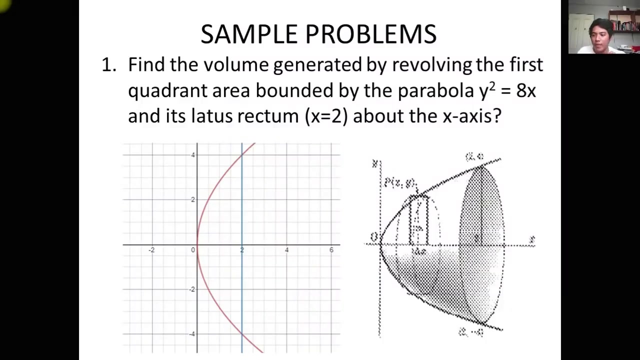 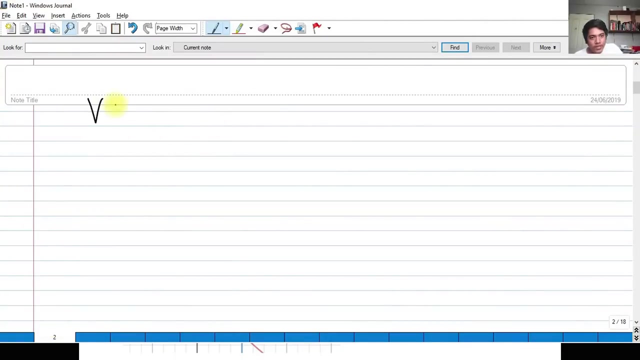 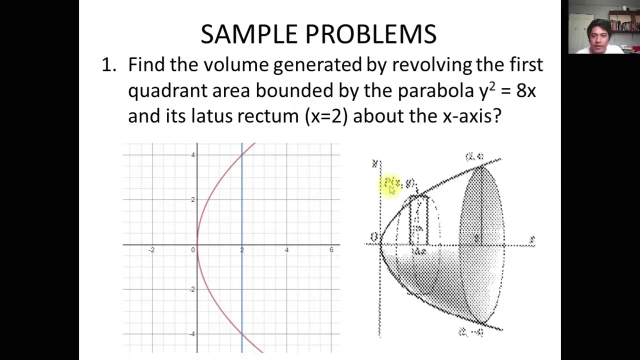 so we are concerned only with the first quadrant here so and then we're going to what to rotate this about the x-axis so if we're going to rotate this about the x-axis we have this figure 3d figure so what what do we mean by x-axis rotation is to rotate it 360 degrees with respect to the x-axis so we have here this revolution so how are we going to find the area of that since we are only dealing with the first quadrant we are going to rotate this about the x-axis so we are going to have to use what so this is a area bounded by one curve and its lattice rectum at x is equals to my mistake this is equal to two so what are we going to do here is simply what use the disc method okay so we have to use the disc method again if the disc method we used to recall we have pi integral of from a to b of y squared dx okay opening or what do you call this axis of rotation is is on the x-axis so for y-axis we have the formula again okay so we have the formula a while ago so this is the disc method y disc method okay disc method so because um we see here that we have a parabola and it is bounded on the x-axis of the line x is equal to two so we can easily use the what the disc method so so volume now will be equal to the 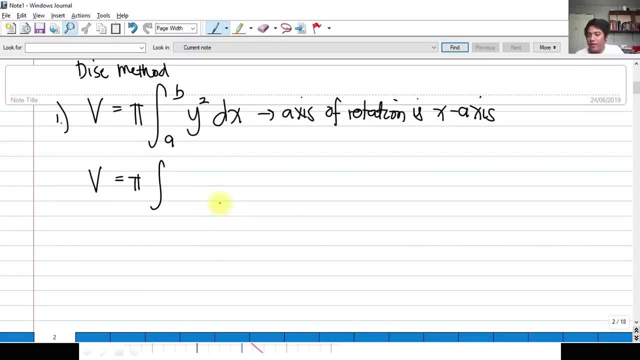 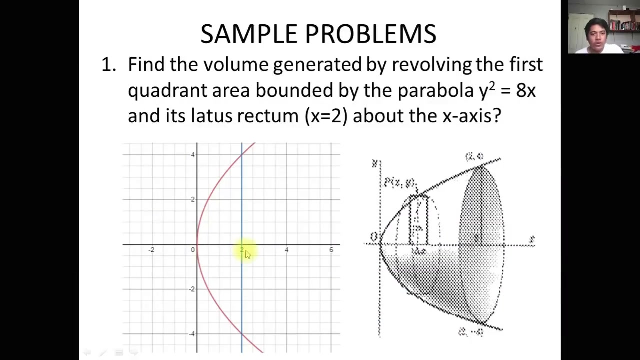 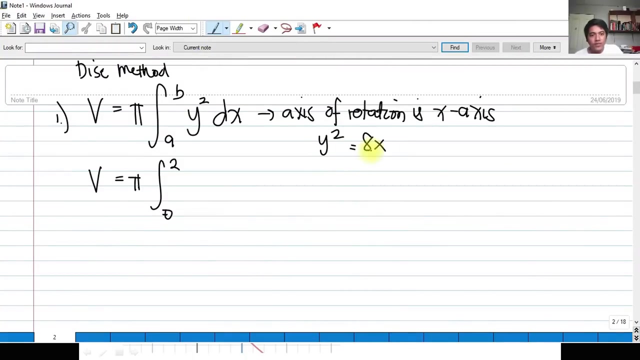 pi the integral okay what are the limits well of course if the limits is its axis rotation is x-axis so the limits should be from zero to two because the lattice rectum we know that the parabola originates from the origin up to two so this will be our unit zero to two okay so zero to two and y squared so and again we have a given parabola y squared is equals to eight x so that would be simply y squared dx so pi integral from zero to two of the y squared and that is equal to eight 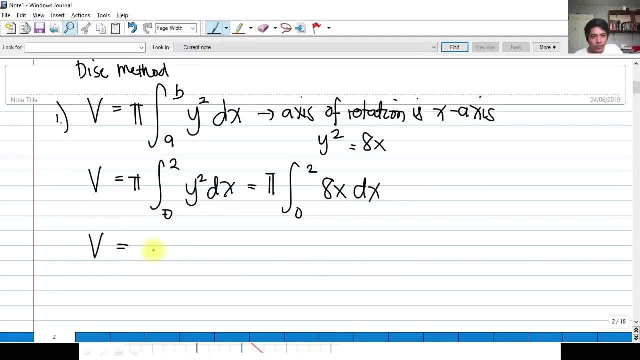 x dx so simply that would be our volume so pi we have to integrate 8x so that becomes 8x squared over two that is 4x okay evaluated from zero to two so we have pi four times uh this is squared 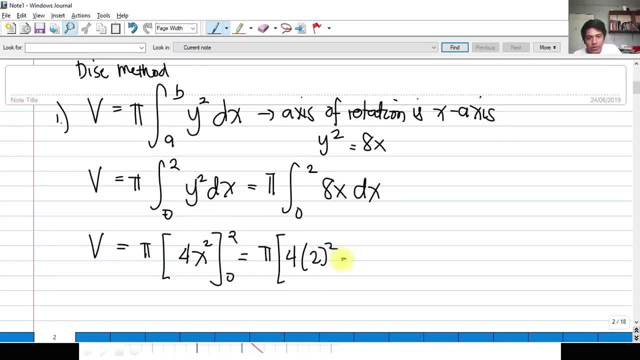 okay four times two squared so minus zero so we have four times four that should be sixteen 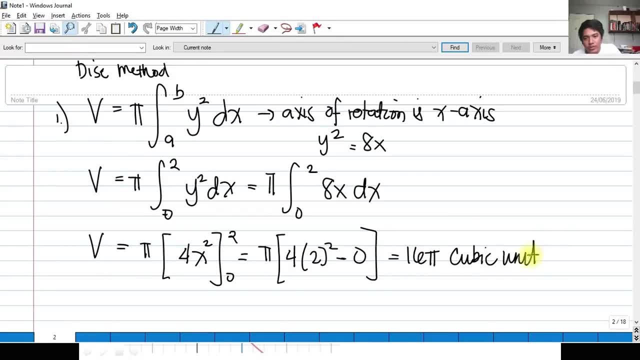 five cubic units again recap of what we have what we need is we use the disc method okay the disc method is actually used when when the curve actually passes through the x-axis boundary okay or y-axis boundary so in this case we have two curves the lattice rectum or x a line and then 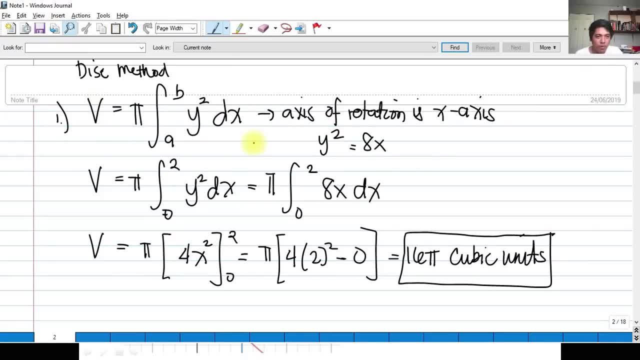 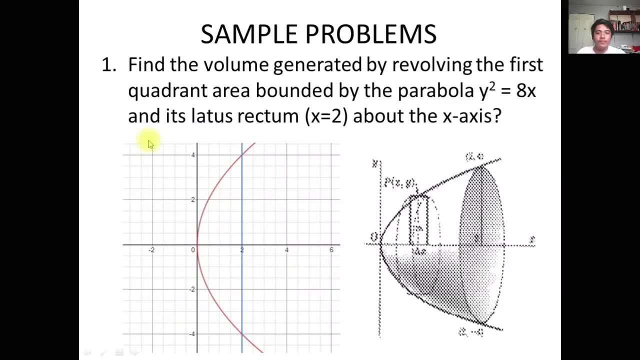 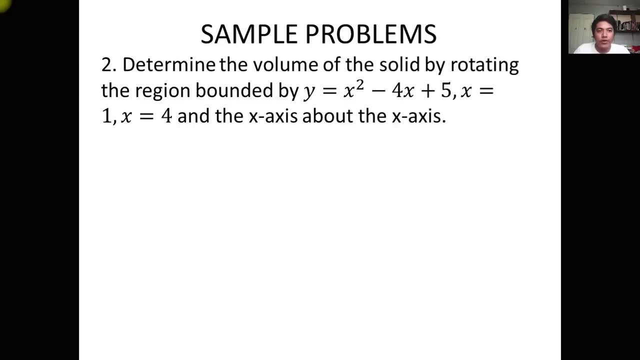 the axis of rotation is x-axis we have used this formula for this method okay so we're done with this okay so for our next problem so we have determined the volume of the solid by rotating 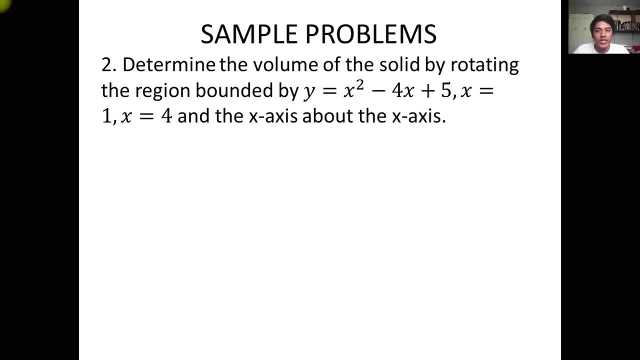 the region bounded by y is equals to x squared minus four x plus five x is equals to one x is equals to four about the x-axis and the x-axis and about the x-axis 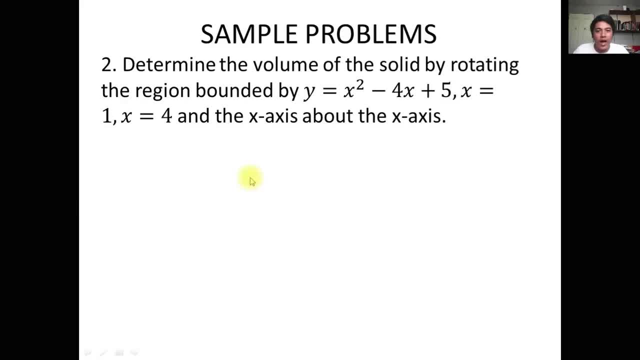 so what is the axis of rotation here we have about the x-axis so still about the x-axis and still we're going to use the disc method here because we have a parabola and bounded by a 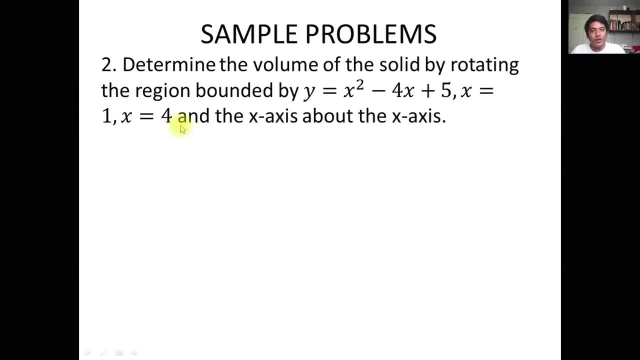 certain point in the x-axis so let's start so again for the next page okay so for number two 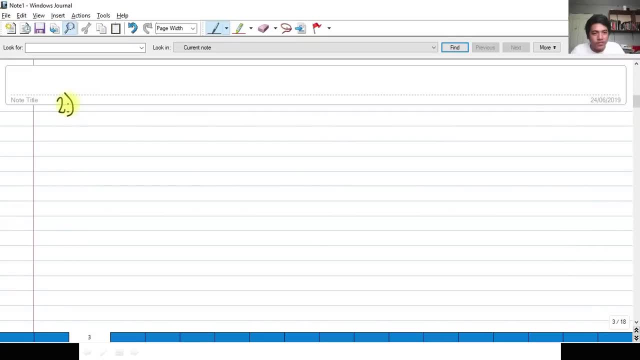 we have the given x squared minus four x plus five so that is y is equals to x squared minus plus five bounded by the x and equals to one and x to four about the x-axis this is the axis of 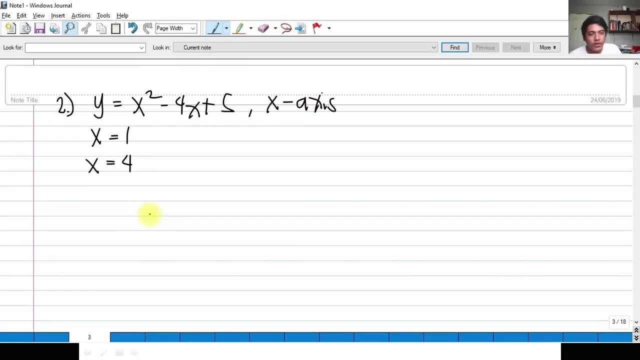 rotation so what are we going to do is first we need to identify the vertices of this parabola okay so we have y minus five okay we have two transposes on the other side so we can complete 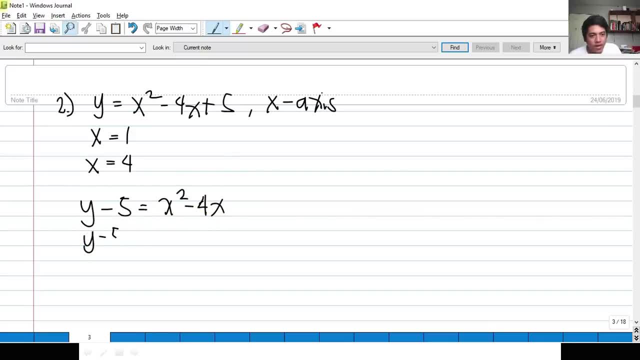 the square of this so we have y minus five is equals to x squared minus four x squared minus four x we have to complete the square plus four so if you add plus four here you have to add plus four here so four plus negative five that is y minus one is equals to x minus two squared so we 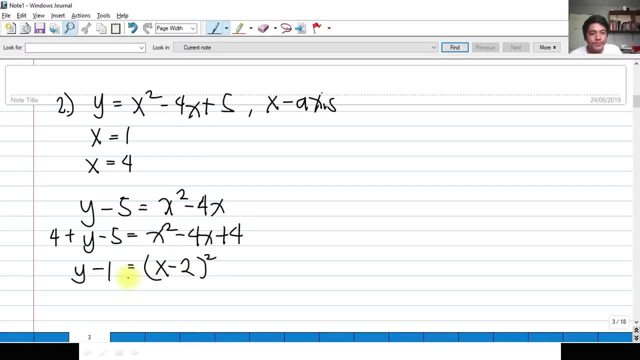 have now a parabola opening what upward so we have the vertex of the parabola as two and what 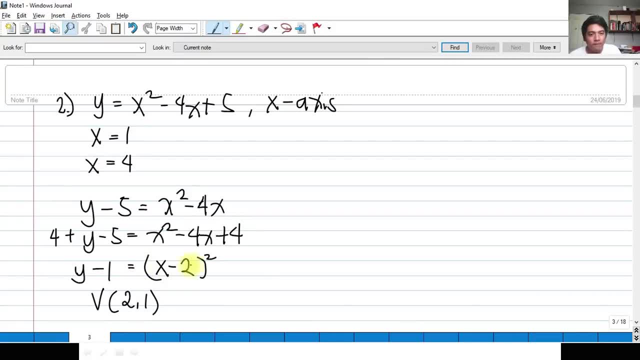 okay so if we wish to draw this parabola we wish to draw this i have a figure here so this is our parabola 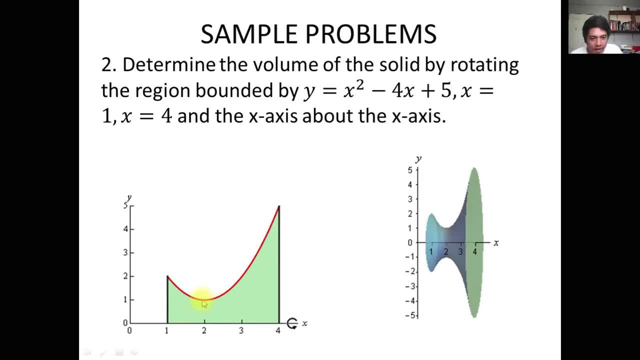 so vertex vertex is in x is equals to two and x y is equals to one so we are we are we have the correct graph so but our concern is only we need to find volume bounded by this parabola with 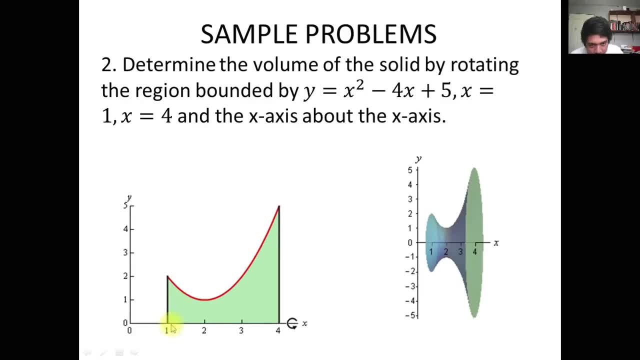 respect to the do the line x is equals to one on the x-axis and x is equal to two on the x-axis is equal to 4 on the x-axis so what are we going to do and again this is about the x-axis or we're going to rotate the this figure with respect to x-axis so after rotation this 2d figure will now 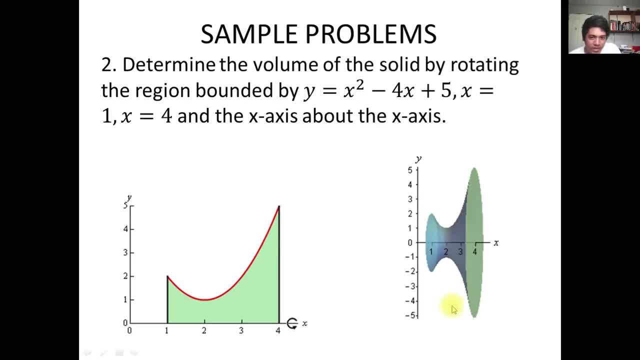 become like this okay it's hard at first to imagine but it would look like this if you rotate this plane 360 degrees this will become the uh this will be the figure now okay and of course 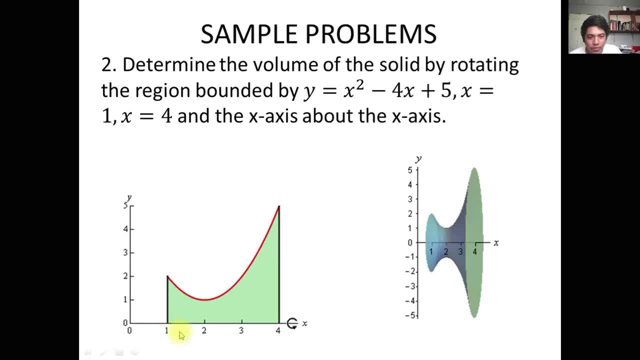 what method are we going to use since this is a parabola bounded purely on the x-axis it has a boundary on x-axis so we still have to use the what the disc method okay so we're going to have 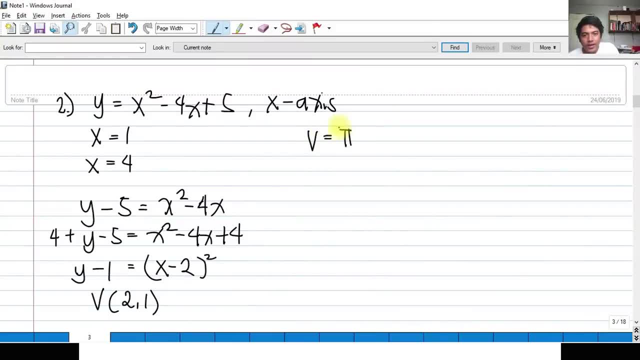 the disc method here the volume would be pi integral of from a to b of y squared dx and again its axis of rotation is on the x that's y dx 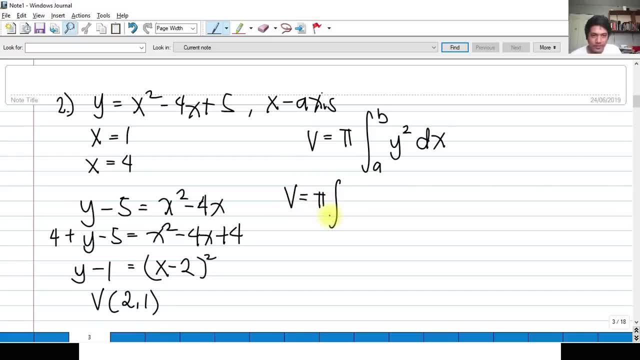 so we have b pi so what are the limits of this it's obvious it's given 1 to 4 so limits from 1 to 4 and we have y squared so what is y squared since if this is y we have to square this so x squared minus 4x 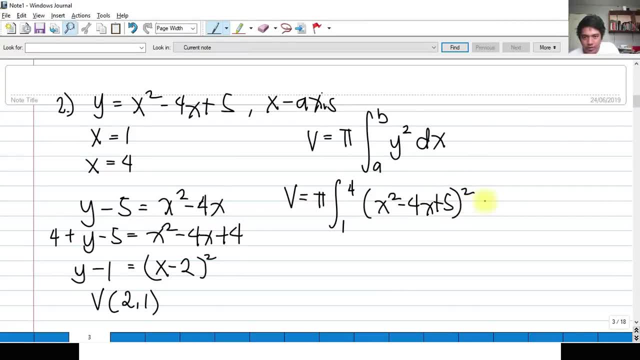 plus 5 squared and that is in terms of the x so how do we square this simply if we square this we will we will have an equal of you cannot foil this you have to uh multiply this on its own so we have x to the fourth x to the fourth minus 8x cubed plus 26 x squared minus 40x plus 25 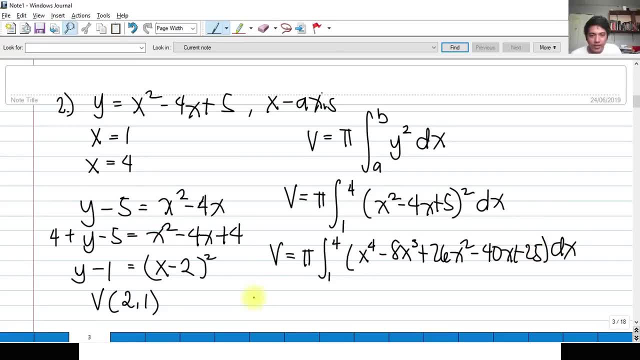 okay uh dx so integrating so we have now the volume is now equal to oops so we have v is equals to pi okay integrate 1 over 5 x raised to 5 so this would become over 4 so 2x raised to 4 plus 26 over 3 x cubed minus 24 per cent plus 25 x squared plus 25 x plus 25 x evaluated from limits word 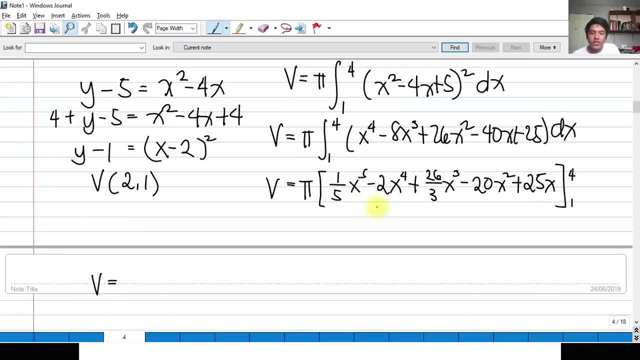 so if we if you evaluate this the volume that you will get so you should know how to evaluate this even this would result to a series of fractions so we know that the result of this integration by the result of this integration by applying the the limits one to four is a number so our answer but here must be 78 over 5 pi cubic units so this would be the volume of the solid of 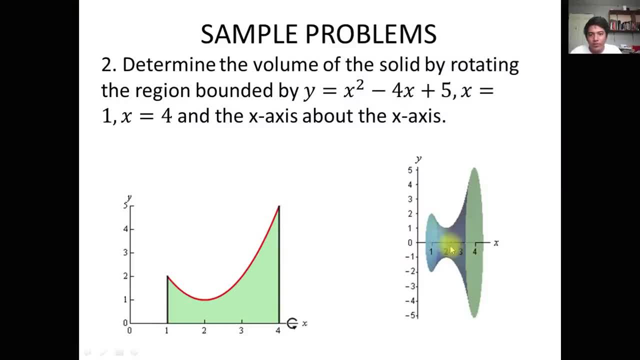 our revolution here so from 1 to 4 so that would be the volume okay so it's kind of hard to imagine at first because it involves 3d dimension but as long as you practice yourself solving some problems involving this so definitely 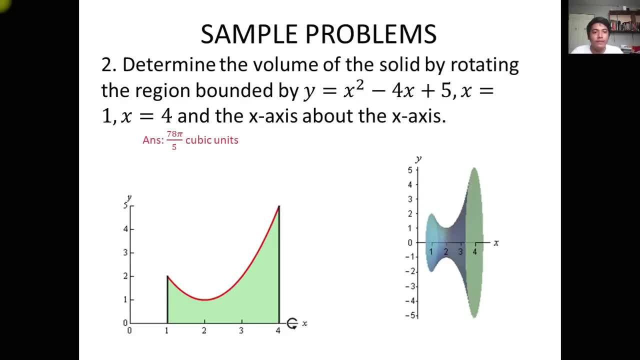 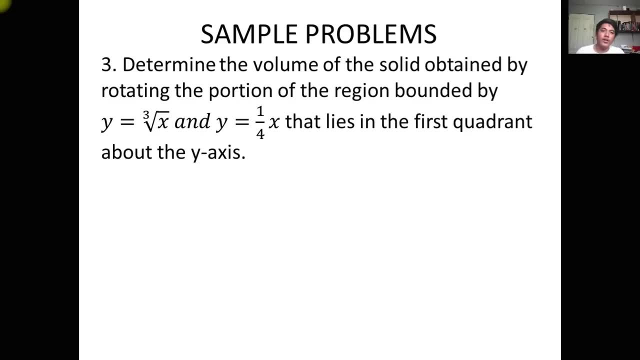 you will be you will get used to it okay so 78 pi over 5 cubic units so for number 3 so determine the volume of solid of 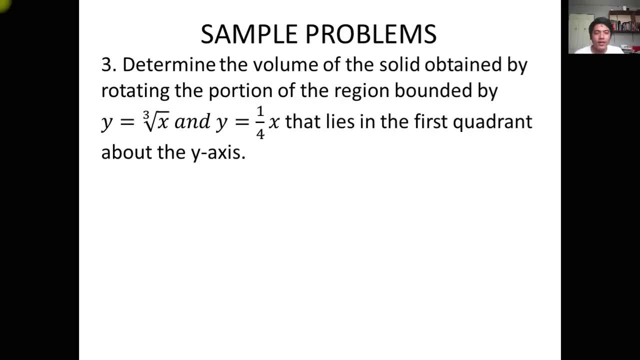 obtained by rotating the portion of the region bounded by Y is equals to cube 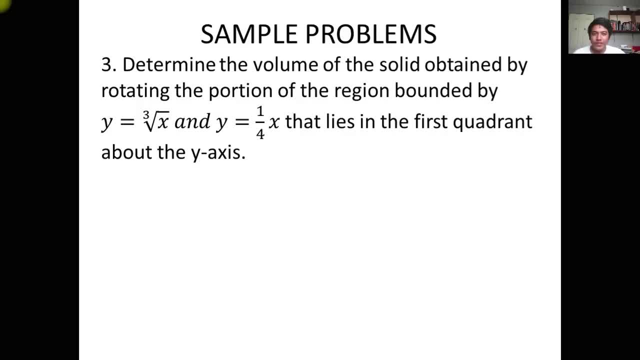 root of X they this is a cubic function and Y is equals to 1 over 4 X that lies in the first quadrant about the y-axis so we have two curves Y is equals to cube 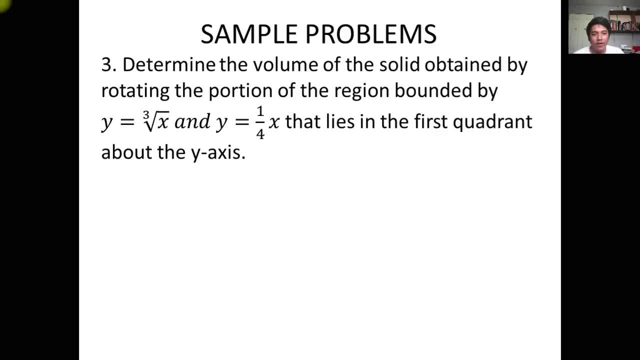 root of X you have to graph it and Y is equals to 1 for X that is a line that 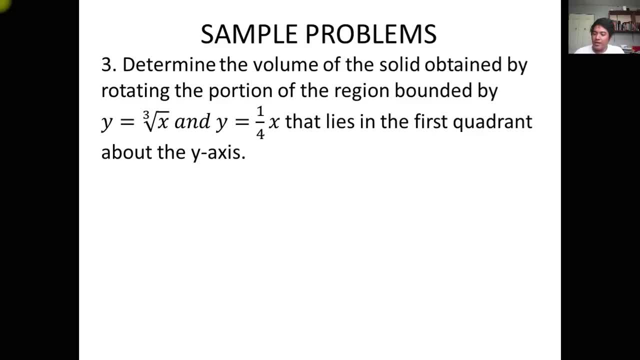 lies in the first quadrant so the problem is only asking the that if we we will 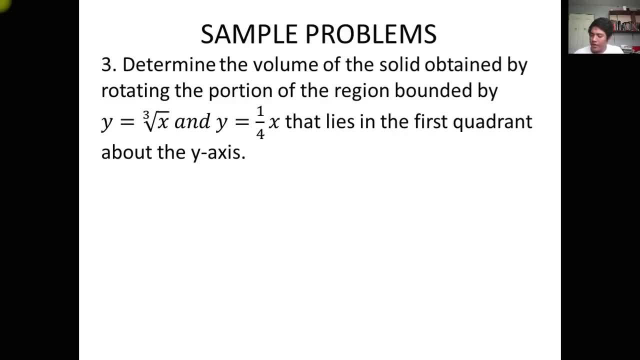 get the volume okay of the the volume of the intersection of these two planes 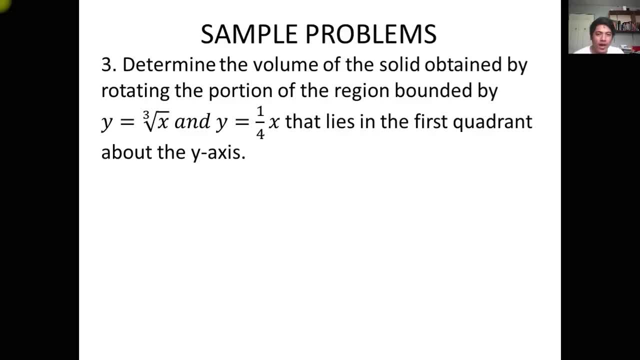 only on the first quadrant about the y-axis so if you wish to grab this so we have this this is the Y is equals to cube root of X okay so or in other words 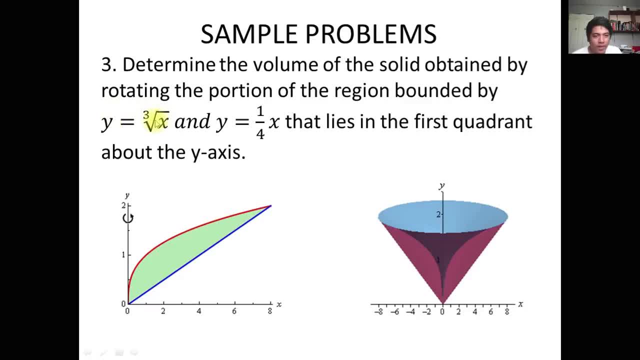 you can simply raise this to 3 so that would become X is equals to Y cube so if your X is actually if your X is if your Y is 1 a your X would be definitely 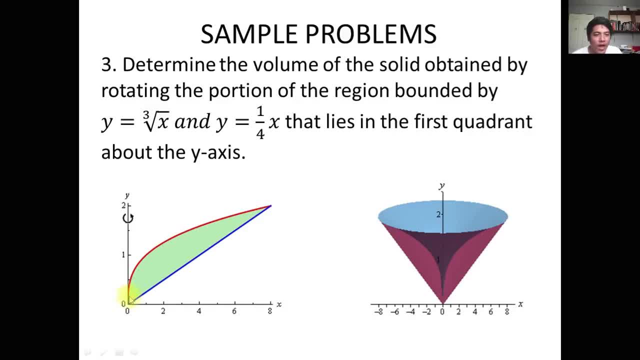 this graph okay so we have this graph and Y is equals to 1 4 over X is here so you we are going to rotate this thing we are going to take this curve about the 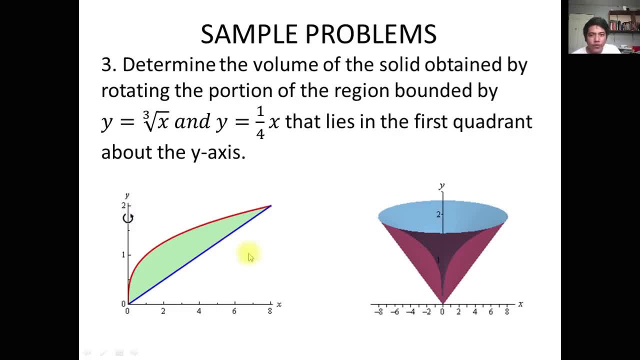 y-axis so we have an axis of rotation so as you can see after rotation this would be the graph so this line okay actually this is the this is our figure first so if you're going to relate this this would be our figure as you can see here 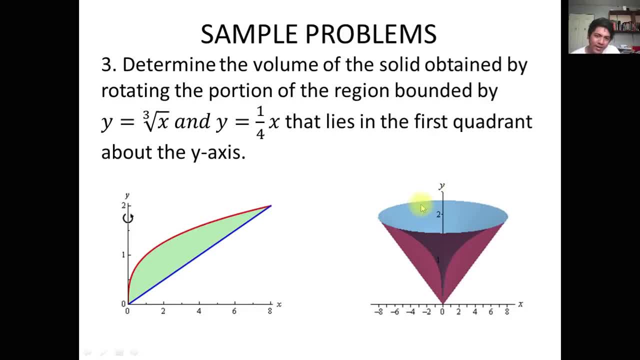 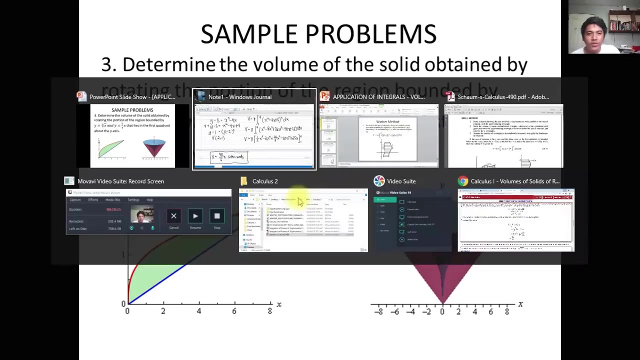 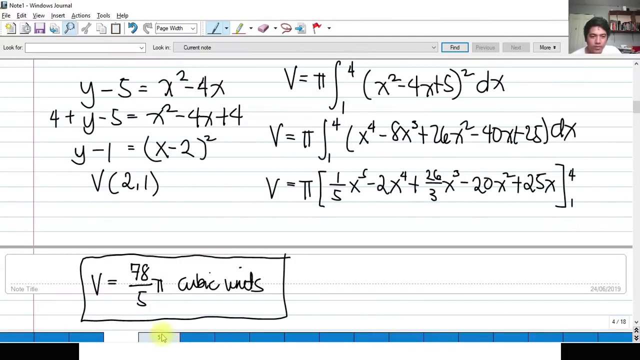 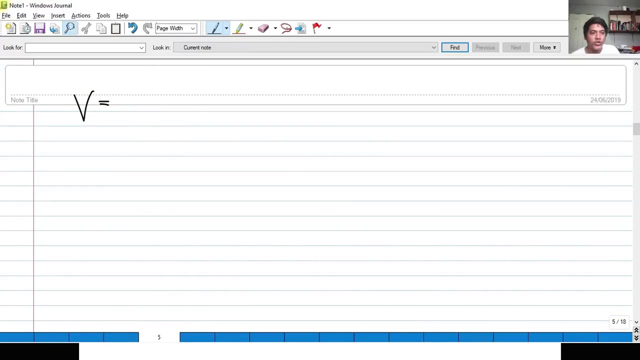 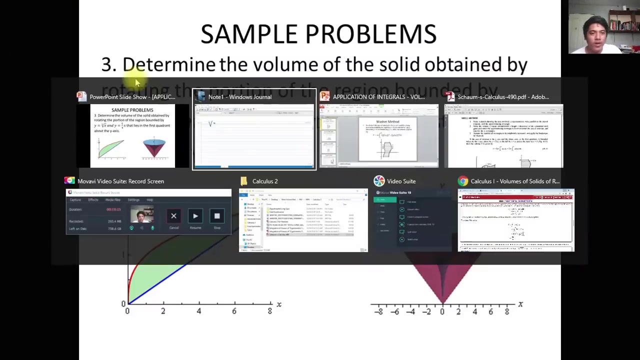 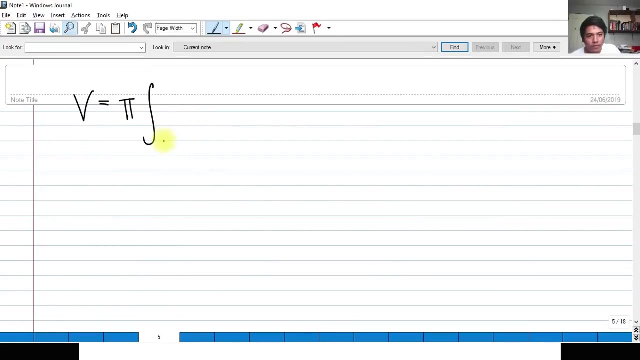 so we have formed a cone but not literally a cone because we have here a cone actually and then we have an inner radius here okay and we have an outer radius here so what are we going to do here is this is not an area or a typical volume that we're going to calculate bounded on the x and y so we have an inner radius here produced by this equation and we have an outer radius here produced by this equation so what are we going to do to get the volume so i've said a while ago we have to use the okay we have to use the we have to use the washer volume washer method so if this is about the y-axis we're going to take it about the y-axis again so our formula would be so our formula would be pi okay the integral of from c to d okay of the f of y squared okay this is in terms of squared minus g of y squared okay in terms of dy because it's axis of rotation in terms of y so as i've said a while ago this is the outer radius outer radius is formed by the washer and this is the inner radius formed by the washer also so we have the volume it's equals to pi okay integral of so what will be the limits what will be the limits well 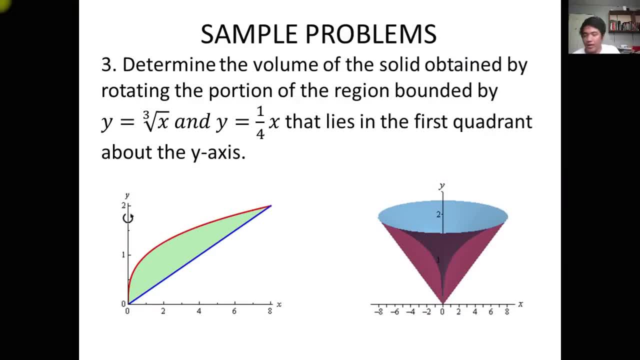 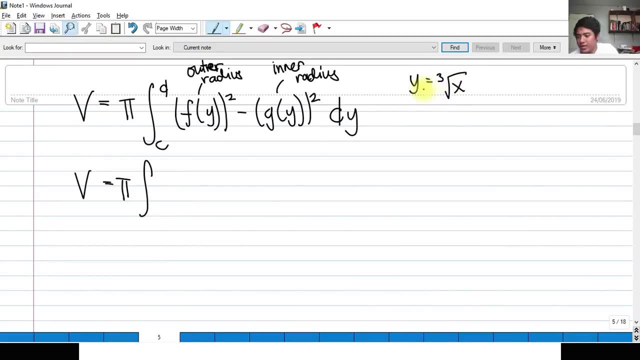 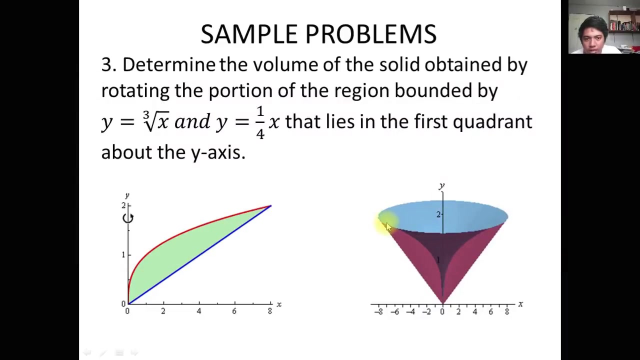 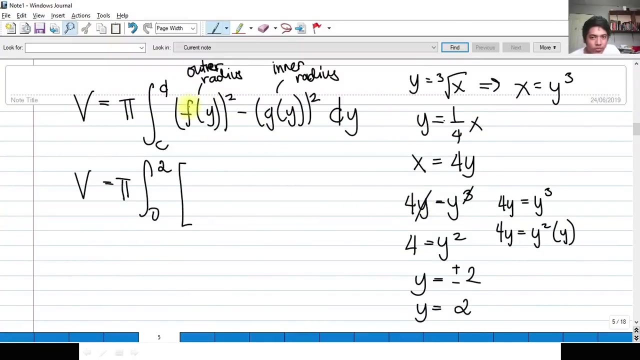 of course we have to determine first what will be the limits of this so our equation is y is equals to cube root of x and we have to express this in terms of y so we have in terms of x i mean minus 8 so we have to have what so x is equals to y cube okay and of course we have y is equals to one fourth of x we have to express this in terms of x so we have x is equals to 4y so if we equate these two we have 4y is equals to y cube so this would cancel actually so we have 4 is equals to y squared and if we evaluate that we have of course positive and negative two but of course we are only dealing with the first quadrant so this should be two only so as you can see here we have what our limits should be from zero to two okay from zero why because we have actually uh this okay and from the figure okay so that should be equal to zero and from the figure it starts from zero the origin okay so that is our limit so outer radius if you are going to look at this graph the outer radius is actually produced by this line okay so this is our outer radius produced by this so if this is the outer radius okay produced by this so it is uh okay to say that we have to express this in terms of y okay so this is our line the outer radius so we have 4 y square that is our line expressed in terms of y okay minus of course the inner radius 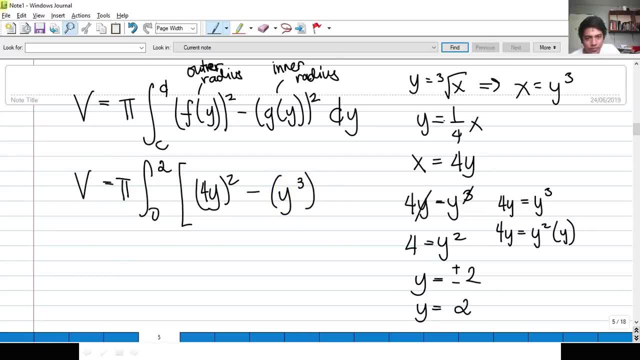 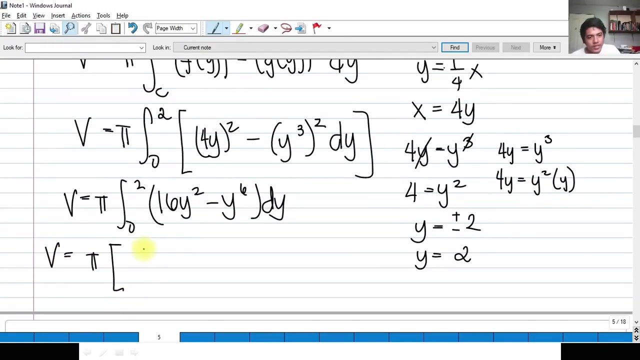 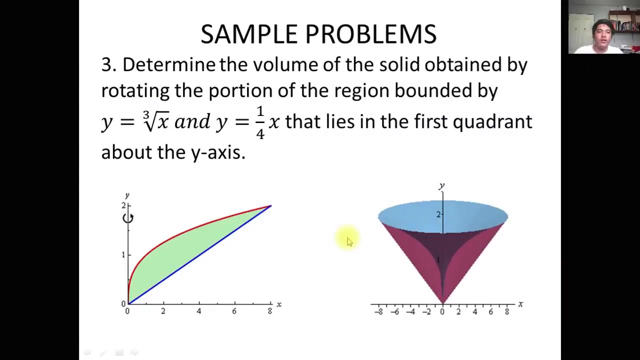 should be the y cube square dy so we got to use the volume this so simplify we have 16 y squared minus y raised to 6 dy and if you calculate that so volume would now be pi 16 over 3 y cube we have already evaluated the integral of this minus 1 over 7 y raised to 7 evaluated from 0 to 2 so if you wish to calculate this so this should be 512 over 21 so the calculation of this is 512 over 21 limits from 0 to 2 multiplied by pi of course we have 5 here so that must be 512 pi over 21 cubic units as you can see here okay for our last problem for today 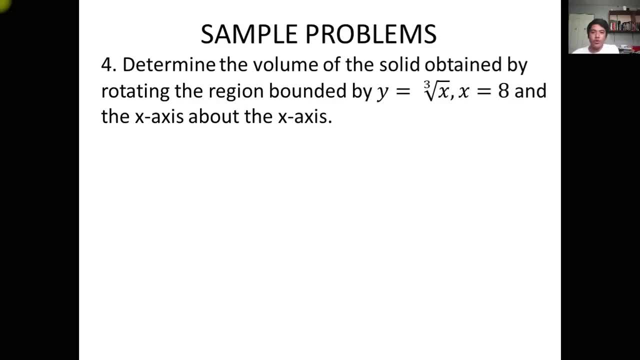 we have the last problem here determine the volume of the solid obtained by rotating the region bounded by steel that's the same graph y is equal to the cube root of x okay and x is equal to 8 and the x-axis about the x-axis so if you wish to graph this again we have a line and a cubic function so first we will be having this this is the cubic function so x is equal to y cube and then bounded by this x is equal to 8 so this is our x is equals to 8 the x-axis about the x-axis meaning we're going to rotate this curve okay to the curve about the x-axis so after rotating we will be producing this 3d 3-dimensional curve 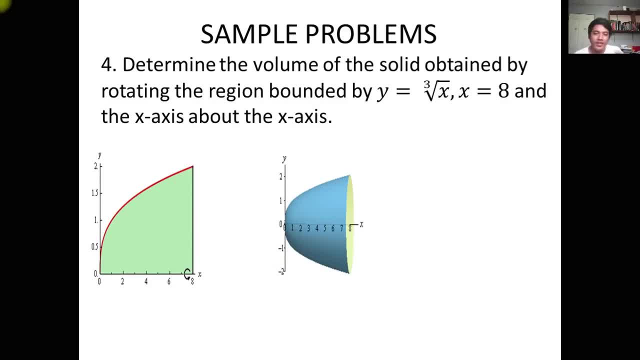 now it looks like a hat or 3d hat so facing to the right this is not a parabola because it's a cubic function 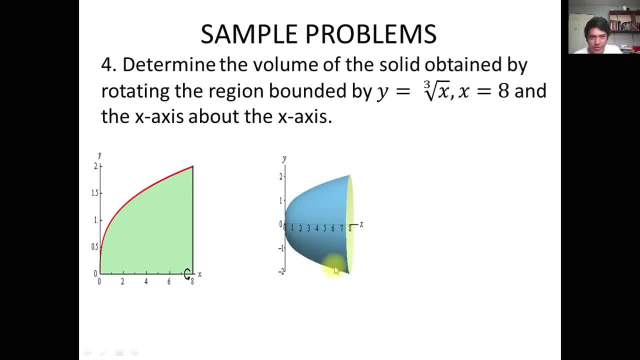 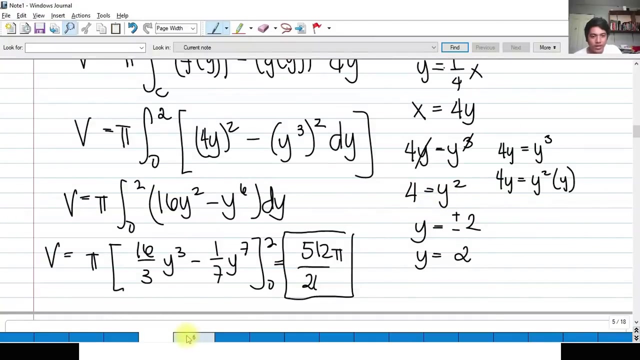 so we have here this figure so uh what do we uh actually need here is to solve this using what the cylindrical uh method so what are we going to do is if we wish to draw a cylinder here okay so we have a cylinder here this is the cubic function and this is x is equals to a so we draw a cylinder here okay in this figure so again if we wish to calculate if we wish to calculate the volume of that through cylindrical method if we're going to recall volume for the 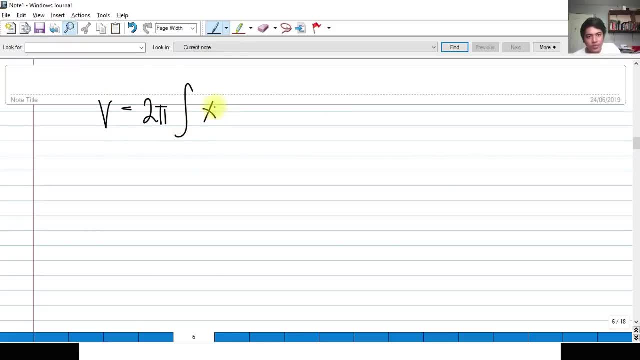 method should be 2 pi x y okay dy if this is rotated about the x axis okay from a to b and volume is equals to 2 pi integral integral of from c from c to d x y dx if this is in terms of axis of rotation of y axis so in this case we 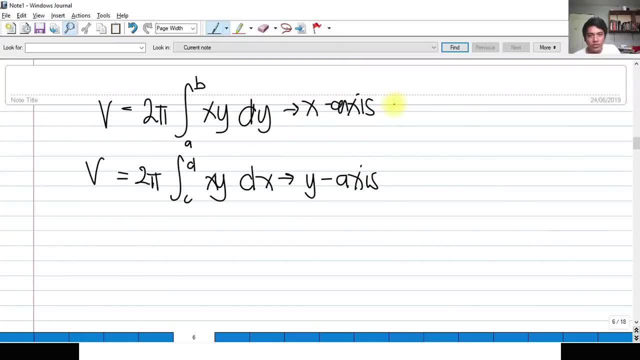 have the axis of rotation is x axis so we're going to use this formula so what do we need b is equals to 2 pi right integral from x y d y now for now that is for now so what would be our limits okay if our if this is dy so we should get the limits in terms of y 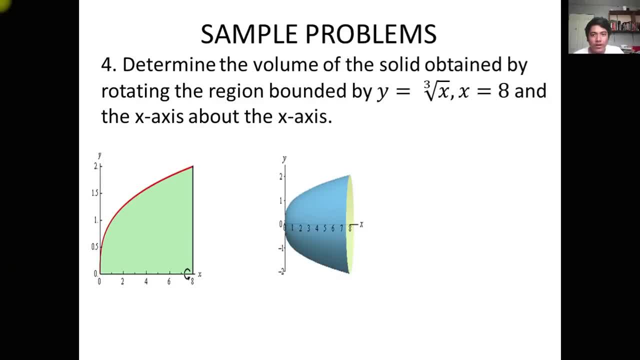 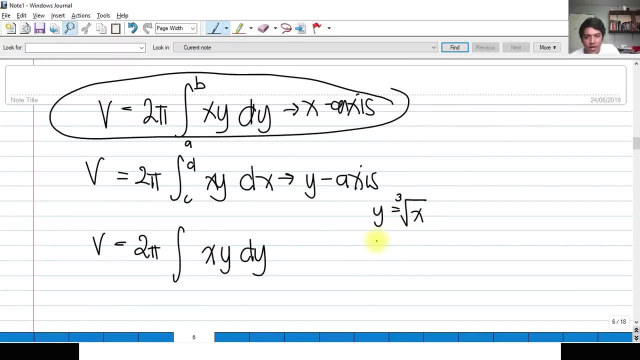 so the height so what are we going to do here again is to what we need to do right so what we are going to do is we are going to 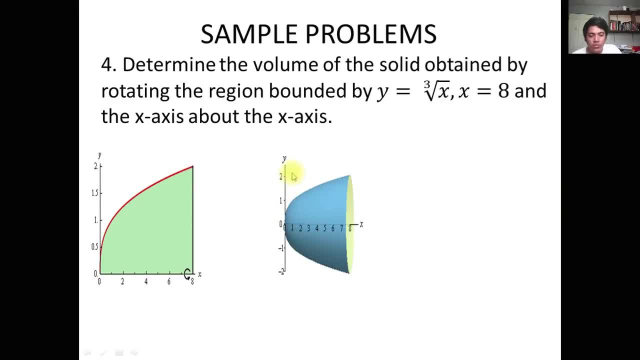 so From 0 to 2. 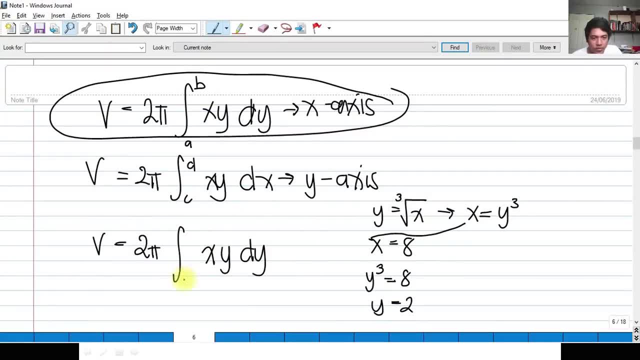 So, and again, we have proven this using the equation. So, from 0 to 2. 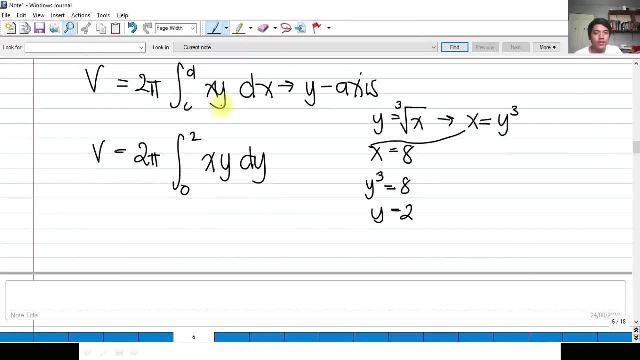 And again, what did I say a while ago about this xy here? This 2xy. 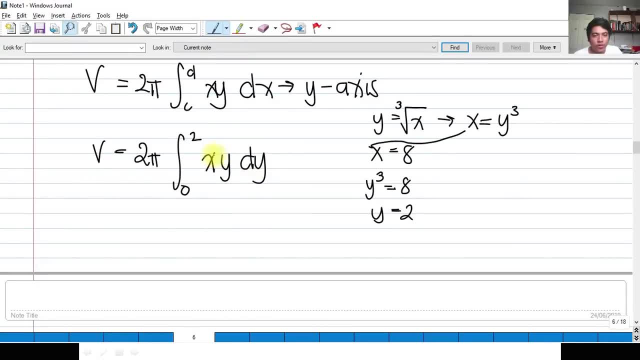 So, we can represent all of this in terms of y. We should represent all of this in terms of y. So, this could be the radius of the cylinder. And y should be the height of the cylinder. 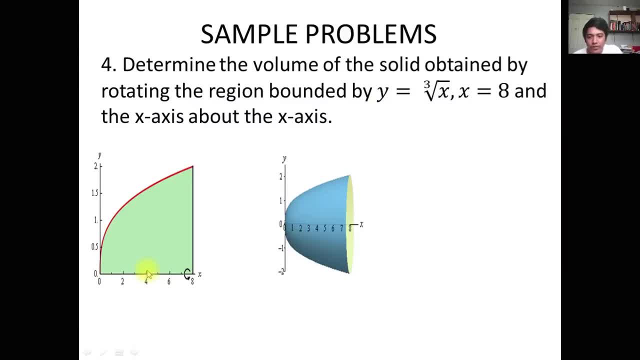 So, back from the figure again. Back from the figure. 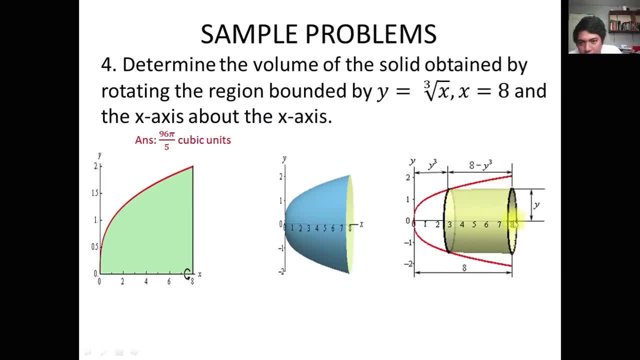 When we have inputted a cylinder here, its radius from here to here is in terms of, of course, y. So, how about the height? This height of the cylinder. So, we know that from the origin to this point of the cylinder, that is 8 because of the x is equal to 8. 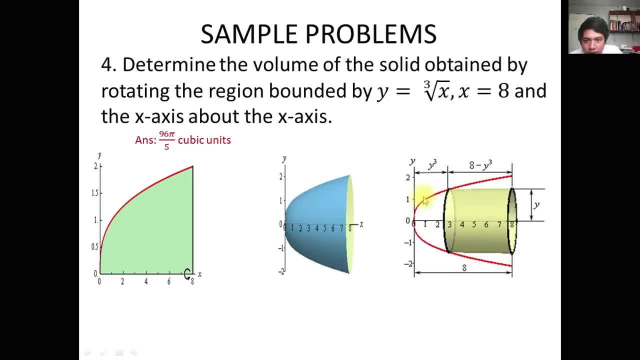 And we know also that this graph from here to here is actually the yq. In terms of y. So, if we wish to get this length or this height of the cylinder, this is 8, this is yq. So, we have to subtract it from the other. So, we have 8 minus yq. So, that if we're going to add this, 8 minus yq plus yq, it would be 8. Okay? So, our height is 8 minus yq. 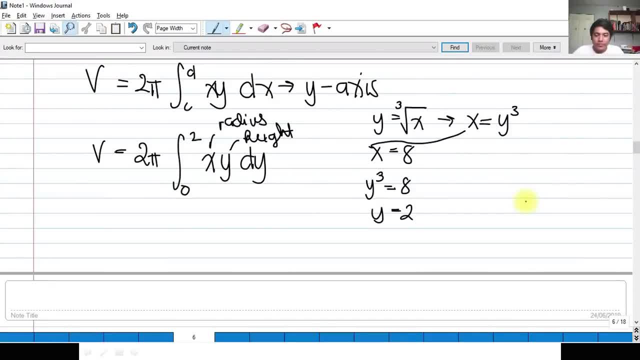 Our radius is only y. So, we can now integrate this. 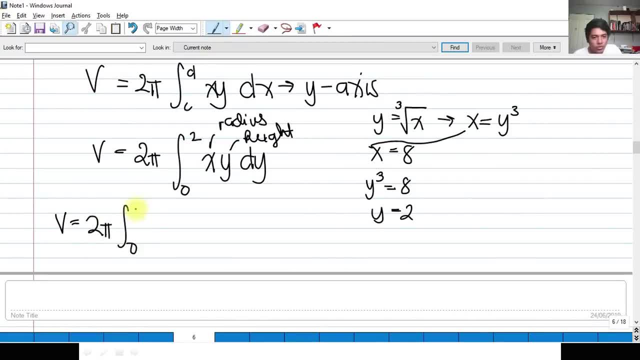 So, v is equal to 2pi integral from 0 to 2. Okay? 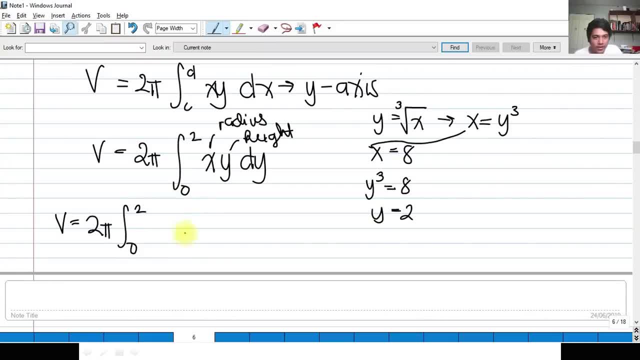 Our radius, again, our radius is y. Okay? 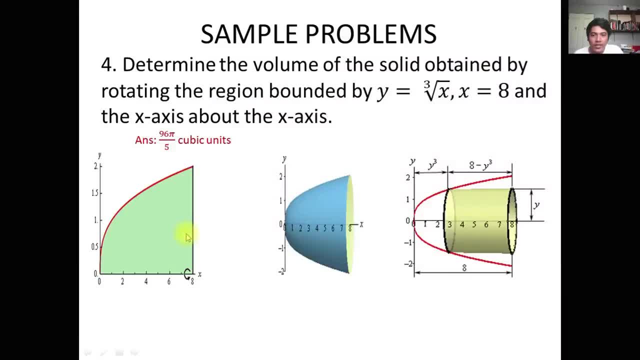 And our height is, in terms of y, is 8 minus yq. So, 8 minus yq dy. So, if we're going to solve that, so, v is equal to 2pi from 0 to 2. 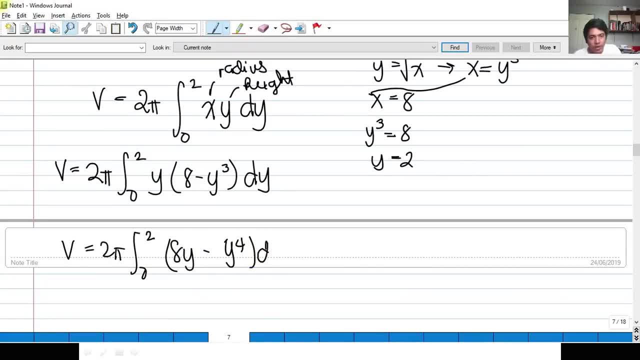 8y minus y raised to 4 dy. Okay? 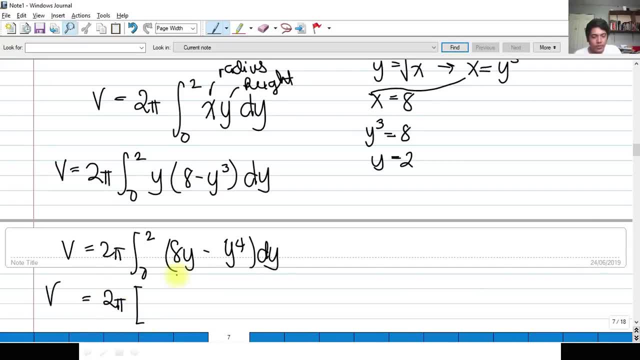 So, the volume would be 2pi. So, we know that 8y2, that would be 4y2 minus 1 fifth of y raised to 5 from 0 to 2. 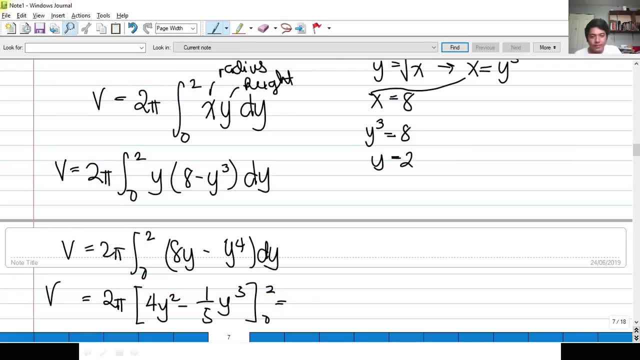 So, if we evaluate that, okay, we shall be getting what? 2 times pi. Okay? Okay. 2pi times this definite integral. 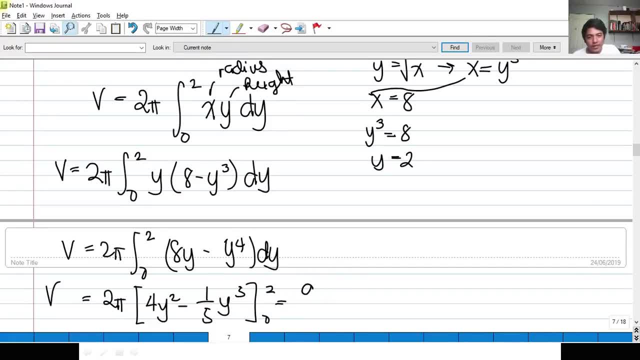 So, you should know how to solve this. So, that would be 96pi. 96pi over 5. And that should be our answer of the volume. Okay? By this. 96pi over 5.